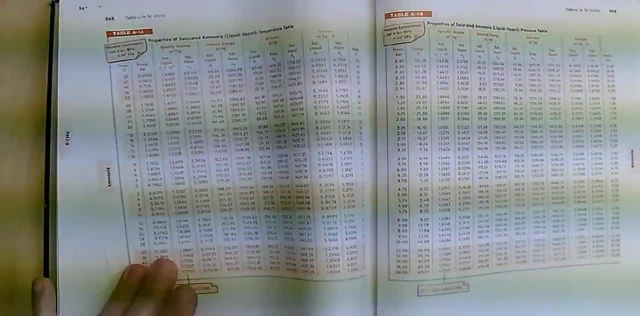 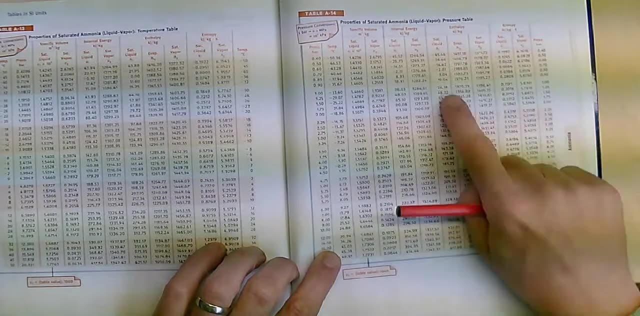 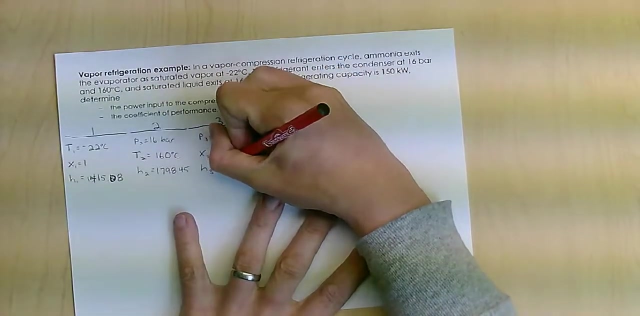 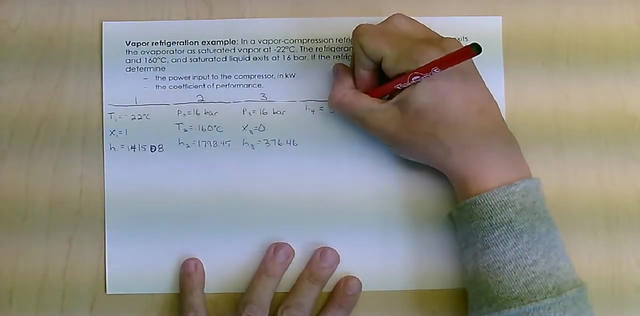 Okay, so then 16 bar saturated liquid. I go back into my saturation table So I'm at 16 bar, which is down here. saturated liquid. I get 376.46, so 376.46.. Now this is the expansion valve, so H is constant across that. so I very easily set my states right here. 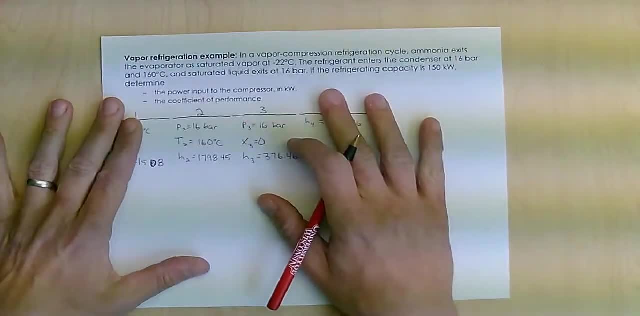 The pressure here is going to be the same as the pressure at 1,, but I don't really need that, okay? So in order to find the power input to the compressor, the first thing I need to do is find my mass. 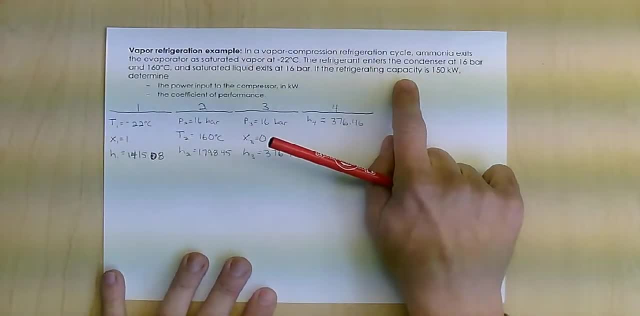 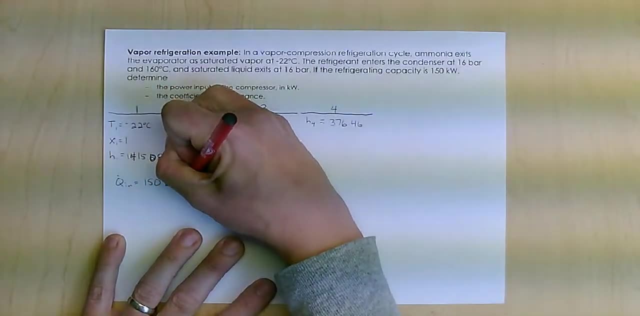 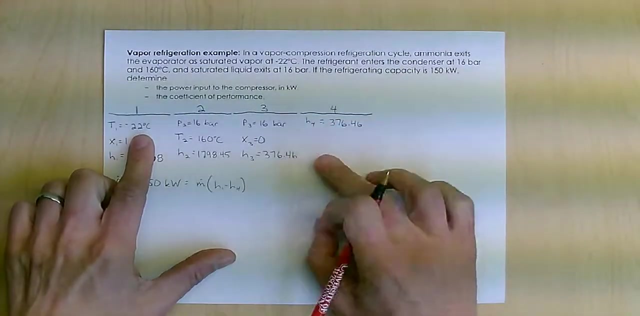 Flow rate- and I can do that using the refrigeration capacity right, which is essentially Qn, which is 150 kilowatts, equals the mass flow rate times H1 minus H4. And again, this is the performance of the refrigerator. this is what's going on. this is what's cooling that space. okay. 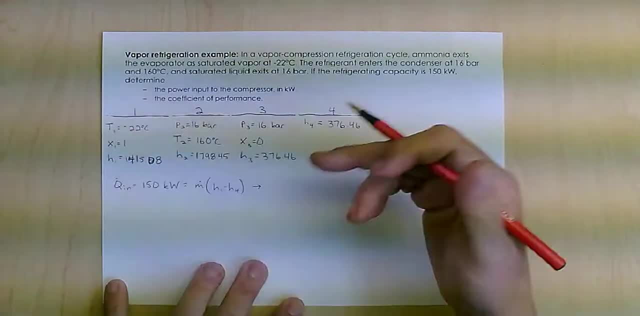 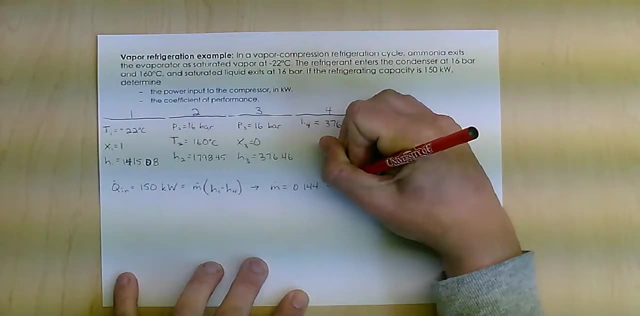 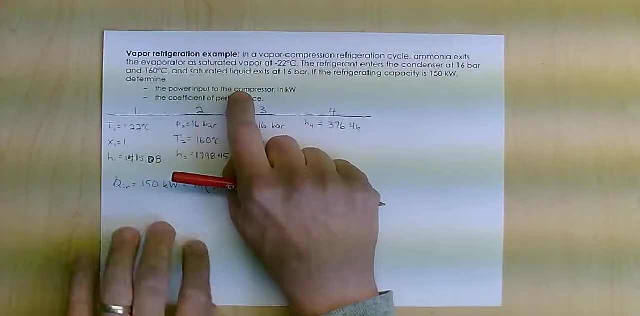 Anyway, from this, knowing H1 and H4,, knowing the refrigeration capacity, I can find the mass flow rate to be 0.144 kilograms per second. okay, Now that I have that mass flow rate, I can go ahead and figure out the power input to the compressor, which again is 1 to 2.. 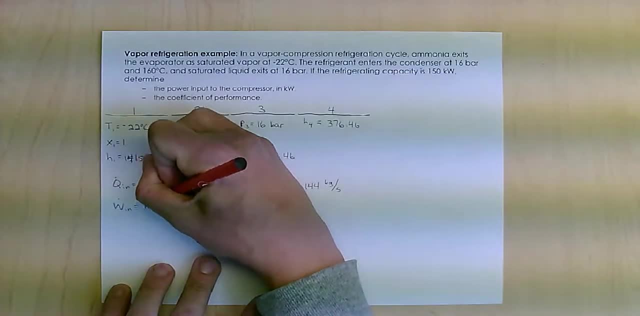 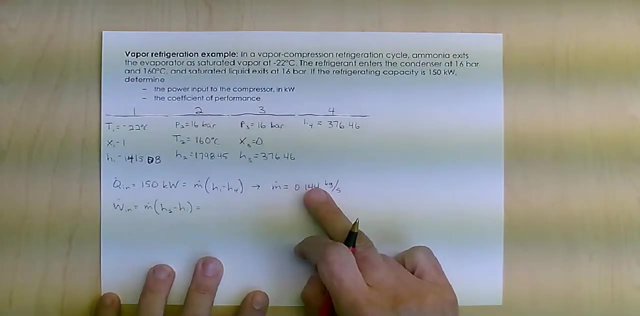 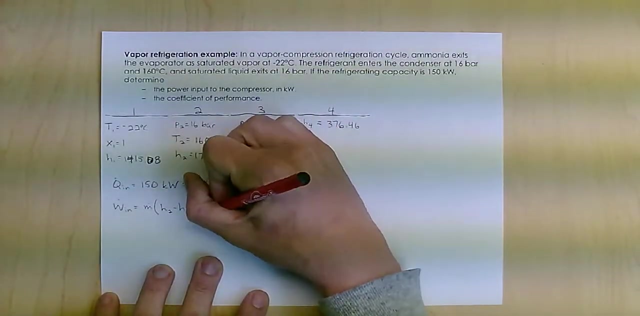 So the input is that mass flow rate. I just calculated times H2 minus H1.. Again, I know H1, H2, I now know my mass flow rate. I can very easily calculate the work to the compressor, Which is 55.4 kilowatts. 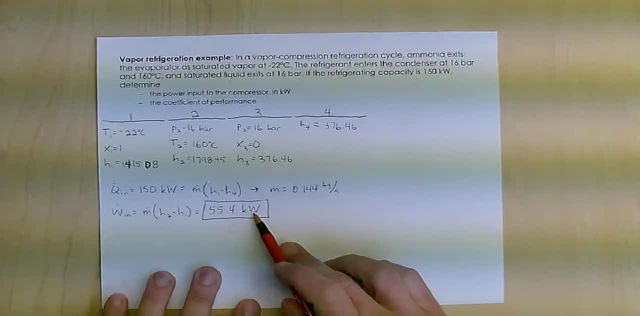 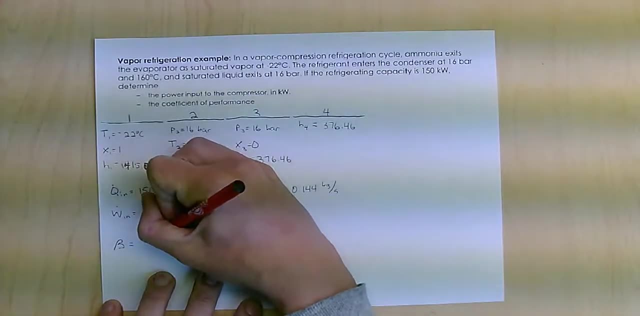 So that's how much power is supplied to the compressor. okay, Now the coefficient performance beta, of course, is output over input. And again, my output is the refrigeration capacity, Qn, which is 150.. My input is the work to the compressor, Wn. 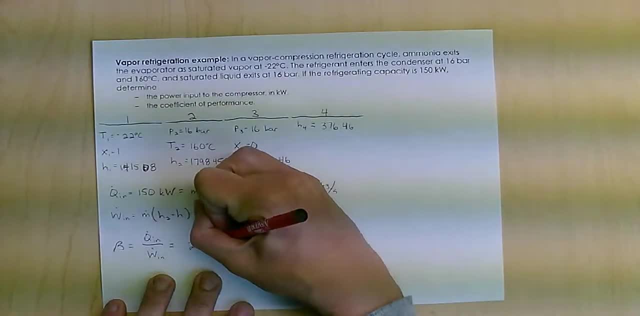 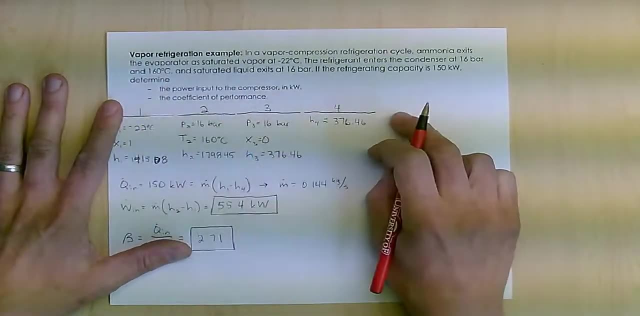 Therefore, I get 2.71 to be the refrigeration Or, I'm sorry, The coefficient performance. okay, So again, as with every problem, go through, set your states. Once you have your states figure out your mass. 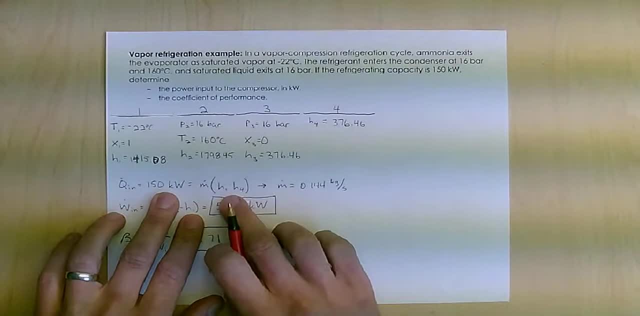 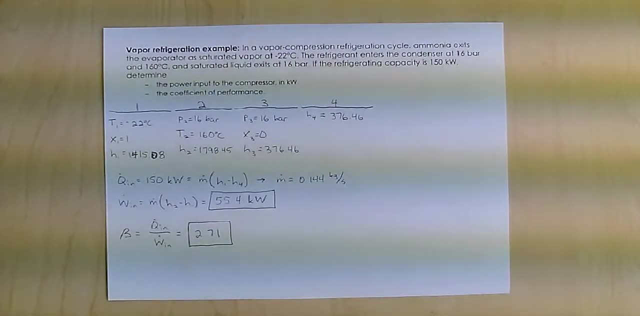 Here I do that. knowing Qn- okay- And knowing my Hs, I can find mass, Then I can find the work to the compressor And then I can find the coefficient of performance.